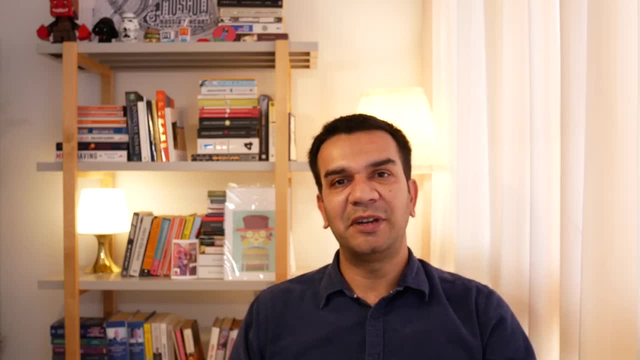 If you like the contents of this video and if you learn something from it, please hit the like button and please subscribe to my channel. I will be posting a lot of similar content and clarifying a lot of other aspects of marketing. In my next video, I will be talking about market and brand penetration in a real world. 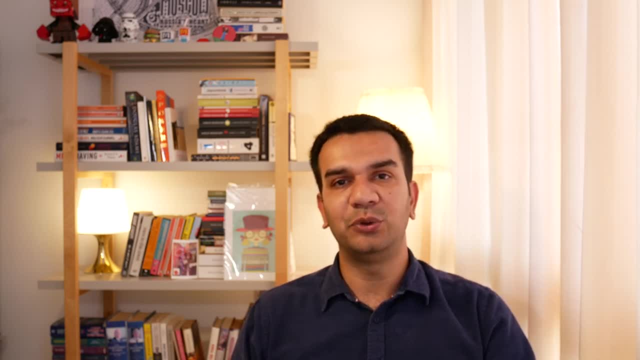 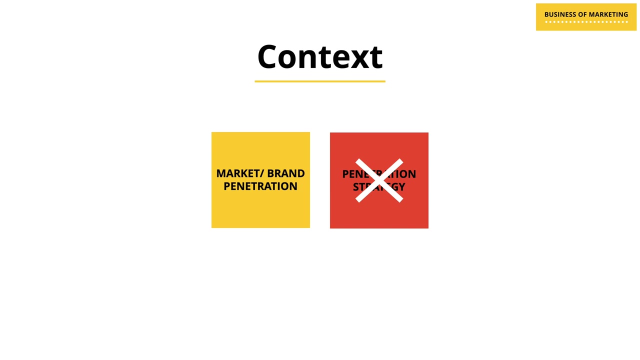 perspective. So please do wait for that and do check it out when it comes out as well. Let me begin by talking about what I am going to cover in today's video. I will be talking about market and brand penetration, and not penetration strategy. 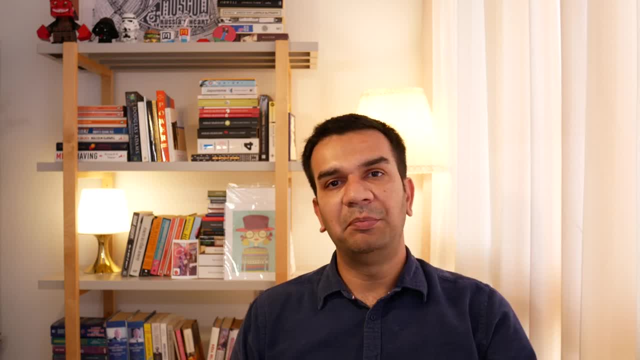 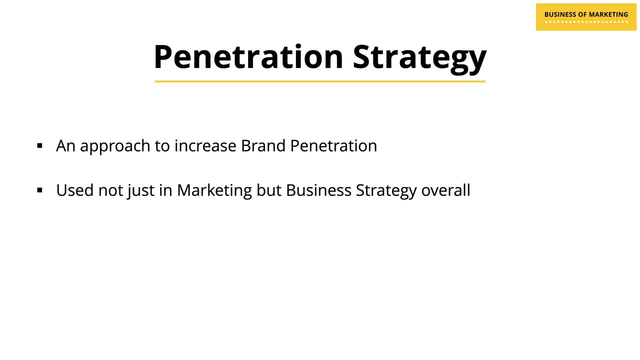 This is the first thing, which is often very confusing. Penetration strategy is something which is not just useful. It is used in marketing, but it is also used in overall business, for strategizing for growth plans and things like that. Market and brand penetration, on the contrary, is something which is like a measurement and 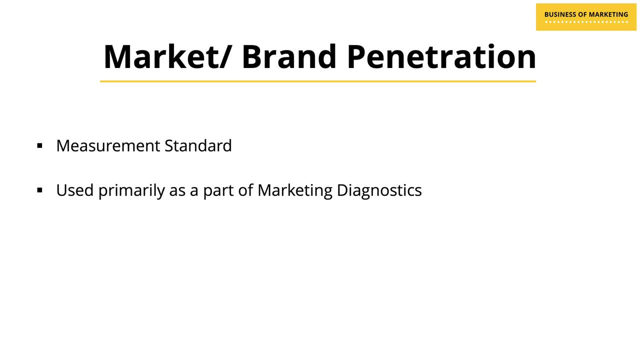 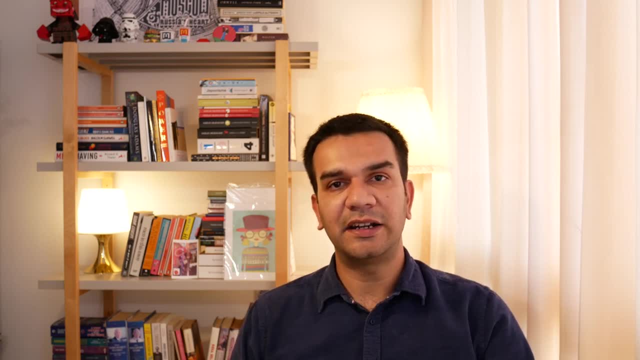 it is a diagnostic tool which is used primarily by the marketers for planning their activities. So I am not going to talk about penetration strategy. I will probably do a different video on that, But in this video I will be talking about market and brand penetration only. 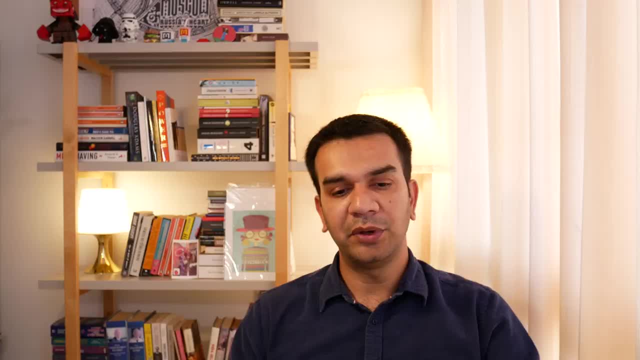 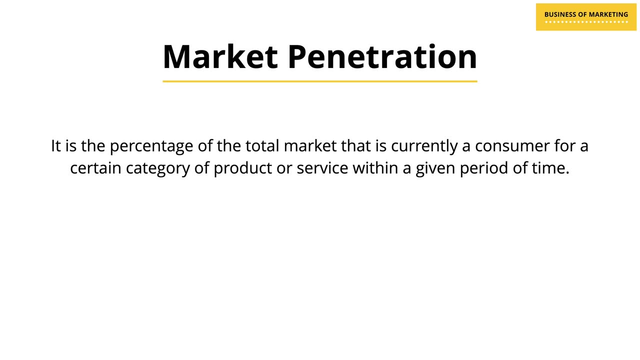 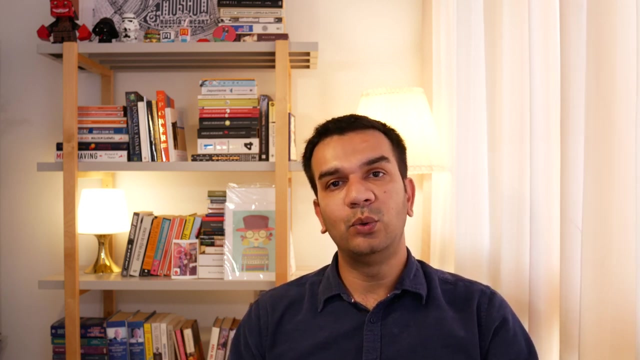 So what exactly is market penetration? I will read it out for you. It is the percentage of total market that is currently a consumer for a certain category of product or service within a given period of time. When we are talking about market penetration, we are relating to people who are currently 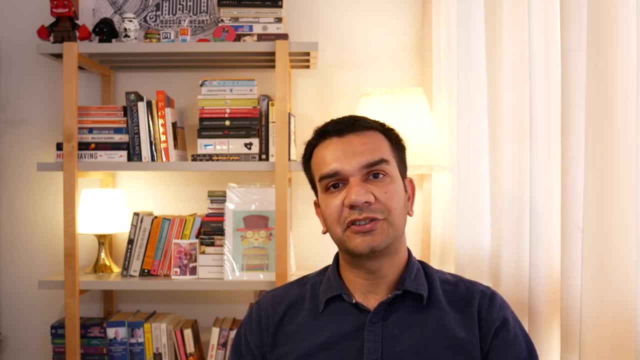 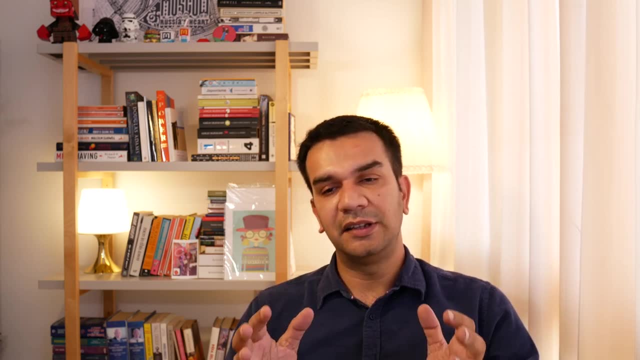 a consumer, Or even when we are talking about brand penetration, we are relating to a specific period of time in a specific place where we have a certain number of customers who are currently buying into that product or service. That is a very important thing to keep in mind. which is currently a consumer? 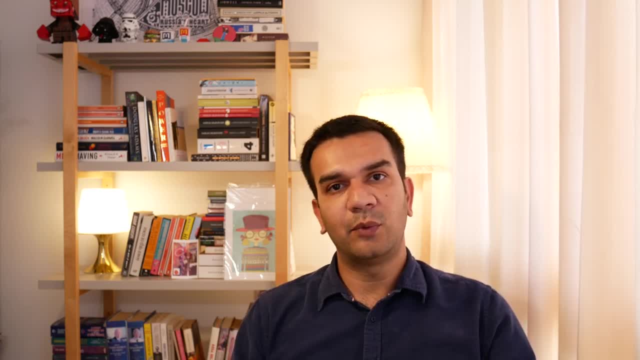 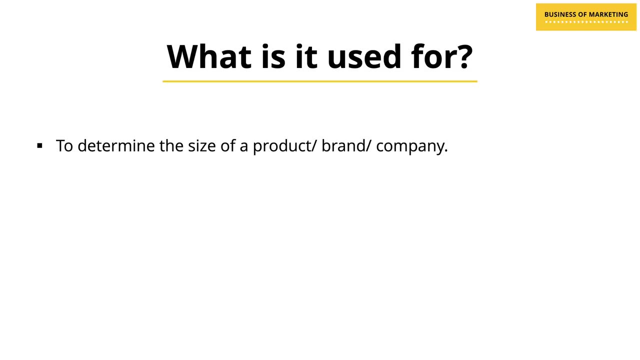 Why is market and brand penetration so important and what is it commonly used for? There are a couple of different things that it is pretty useful for. Some of them are to determine the current size in terms of how many number of consumers that a particular product or a brand or a company has. 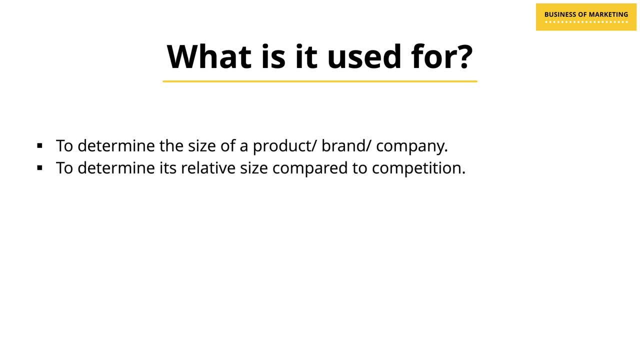 It is also an indicator of the relative size, that what is the size of the competitors, and therefore you can try and understand what is the relative size. It can help you understand how much opportunity exists in the market when you know this kind of data. 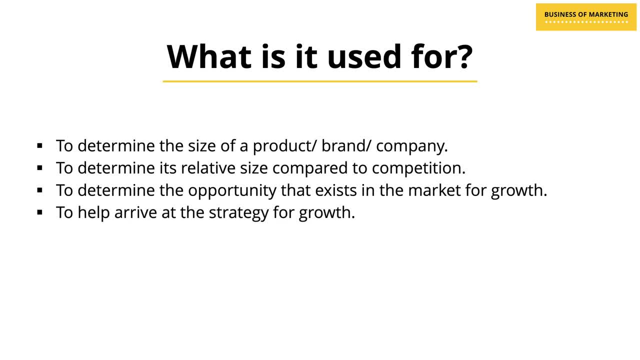 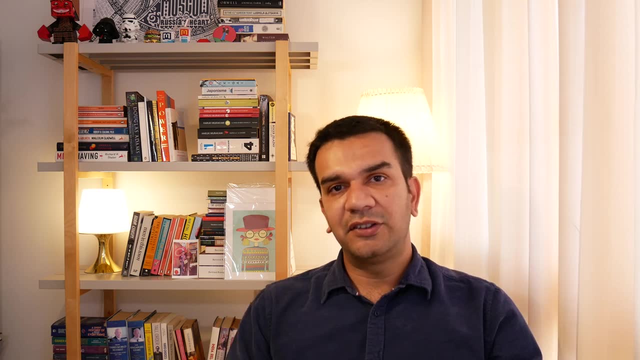 And therefore, using all of this, you can arrive at a penetration strategy Or a growth strategy as to how do you go about tapping into that opportunity that you see in the market. As I was saying, there are a couple of similar terms, so please don't get confused by it. 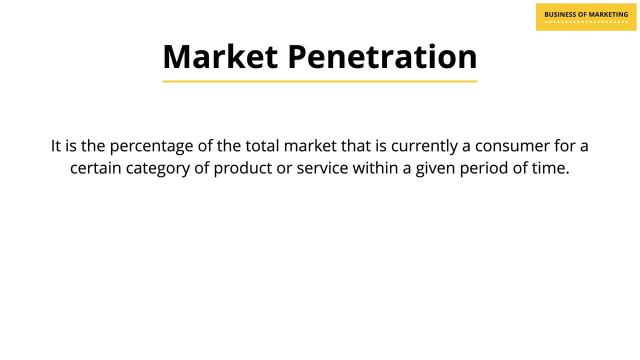 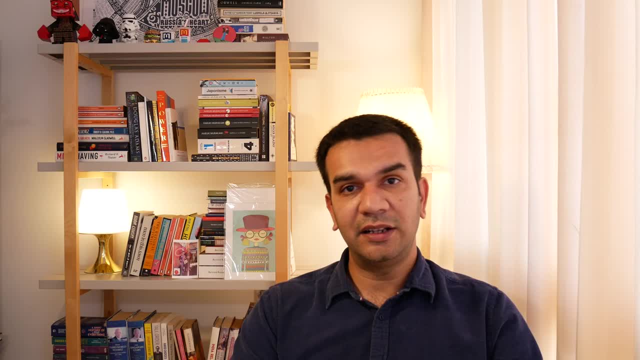 The first one is market penetration- that we have just spoken about, The number of customers of a particular brand or a category currently. The next one that I am going to talk about is market potential. When we talk about market potential, we are referring not just to the number of customers. 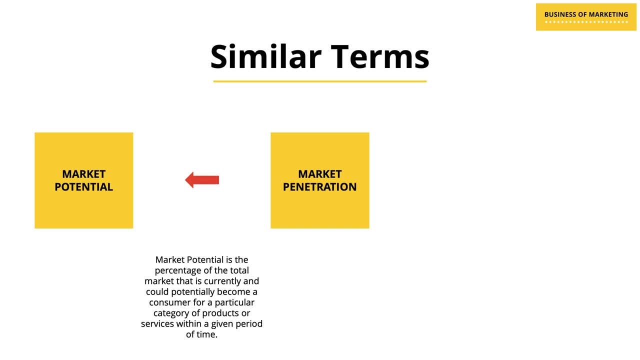 but to the number of customers that are currently buying into a particular brand or a category. The next one that I am going to talk about is market potential. When we talk about market penetration, we are referring not just to the number of customers, but to the number of potential customers or consumers that you can have in a particular 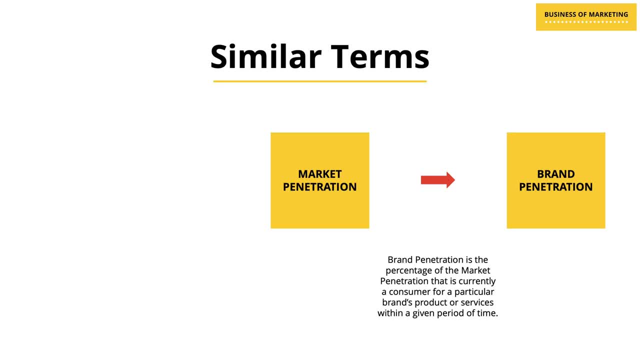 market. The other related term is brand penetration. Market penetration is something which we refer to as for the entire category, But when we are talking about brand penetration, what we mean is the penetration for that particular brand, which is a part of the category penetration. When market penetration is expressed as a percentage, it is called the market penetration rate, And the same is true for brand penetration and market potential. When it is expressed as a percentage, it is called the brand penetration rate or the market potential rate. Let's look at an example to try and understand these different terms a little better. 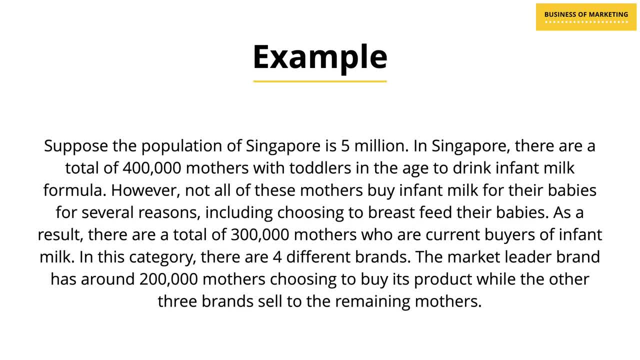 For example, imagine that we are talking about a market which is Singapore, that the population of which is around 5 million. In Singapore, there are a total of 400,000 mothers with toddlers in the age to drink infant milk formula. However, not all of these mothers buy infant milk for their babies, for several reasons. 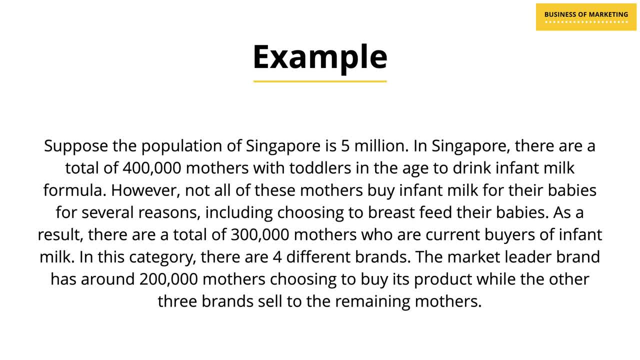 including, say, for example, choosing breast milk to feed their babies. As a result, there are probably a total of 300,000 mothers who are current buyers of infant milk. In this category, there are four different brands and the market leader has around 200,000. 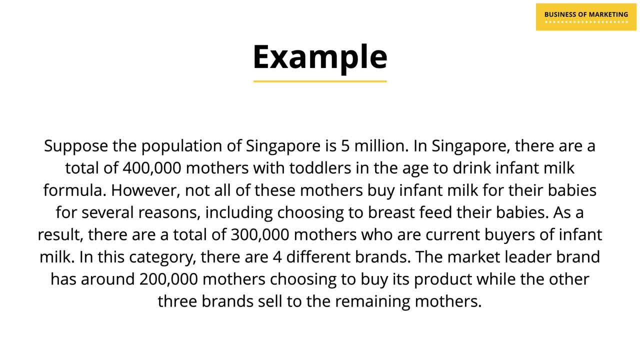 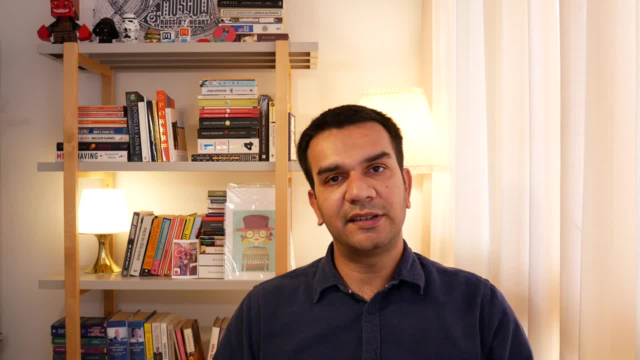 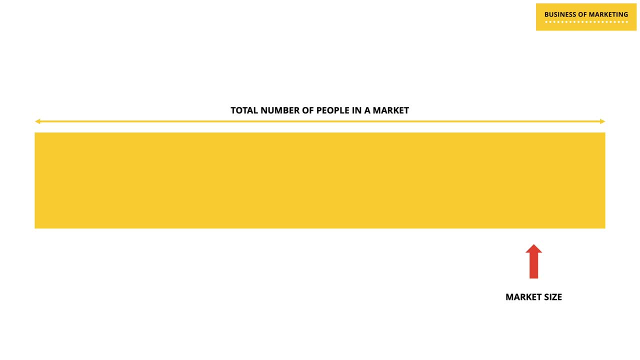 mothers who are currently a consumer of its products. The remaining 100,000 are kind of shared between the remaining three brands. With the help of this example, let's try and understand these terms a little better. So let's first talk about market size. Market size is the total number of people in a market. In our example, we are referring to Singapore as the market. Therefore, the size of the population that we are referring to is 5 million. So therefore, the market size in this example is 5 million. 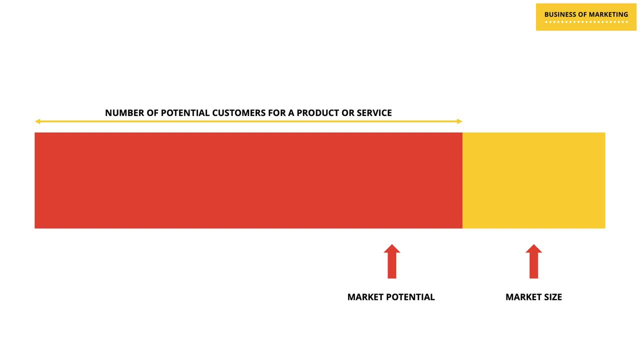 Next, a part of that market size, which is the total number of customers currently, as well as potential customers for a particular product or service, is what is referred to as market potential. So market potential is actually not just people who are already consuming a product or a service. 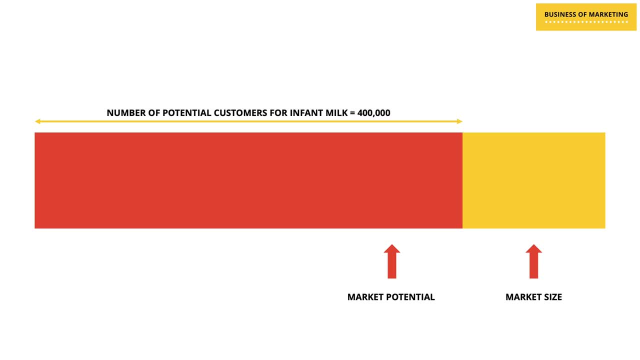 but even those who could potentially consume a product or a service. In our example, the number of potential customers for infant milk is 400,000.. So now that we know the market size as well as the market potential, we can very easily calculate the market potential rate. 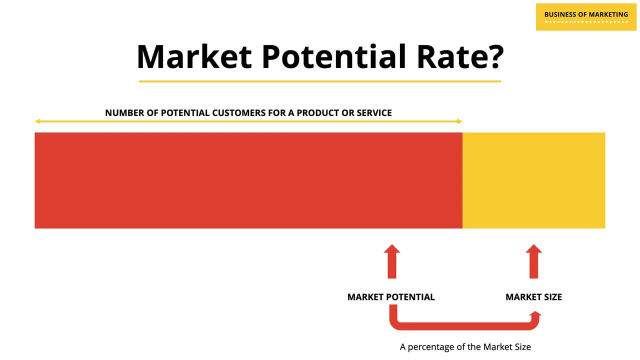 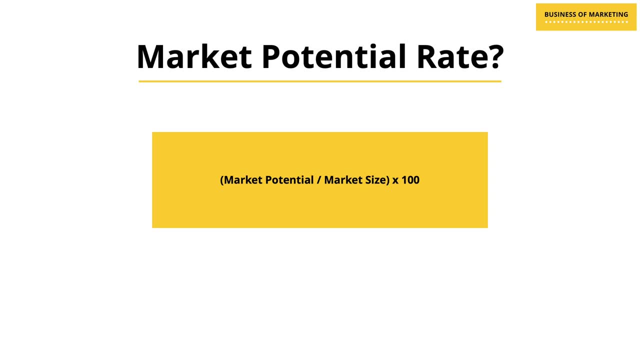 The market potential rate is merely a percentage of the market size. So therefore, in our example, market potential divided by market size into 100 will give you the market potential rate, which is 8%. So in a way we can say that 8% of Singapore market are potential customers for infant. 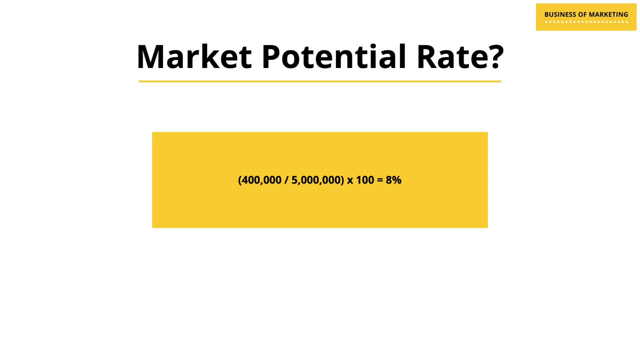 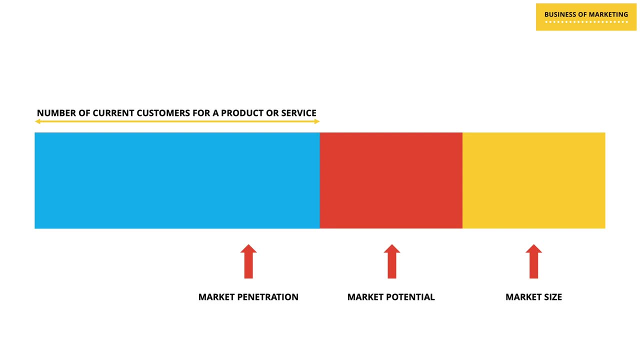 milk in a given period of time. Now let's come to market penetration. We know the size of the market, a part of which is market potential and a part of that is actually market penetration. So, in our example, the number of current infant milk customers. 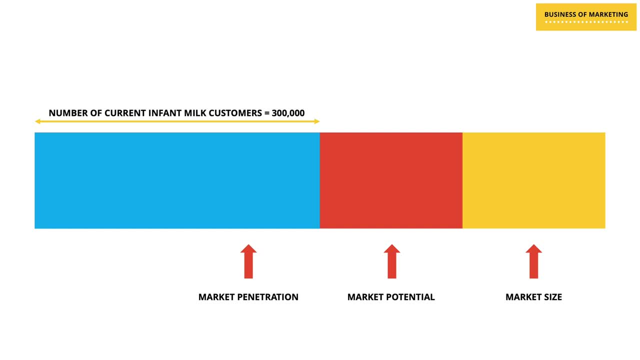 Which is 300,000, is the market penetration. So what we have done is we've basically removed all the potential customers and what we are left with is the actual customers who are currently consuming the infant milk, And that is 300,000.. 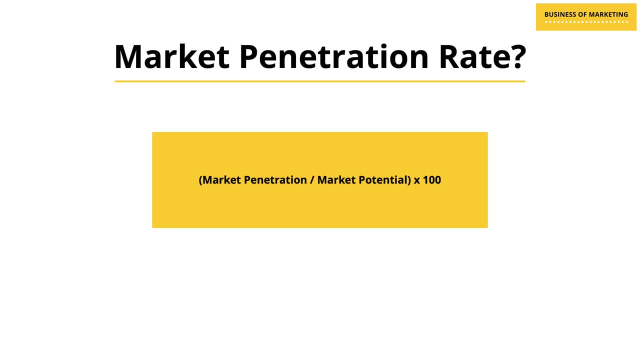 If we were to calculate the market penetration rate, it would be a percentage of market potential And in our example, if we divide market penetration by market potential and multiply that by 100, we will get the market penetration rate, which is 75%. 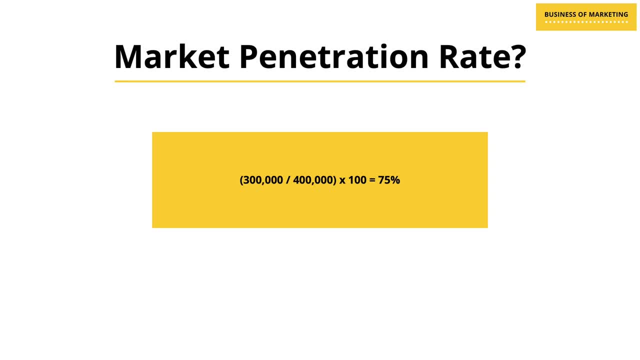 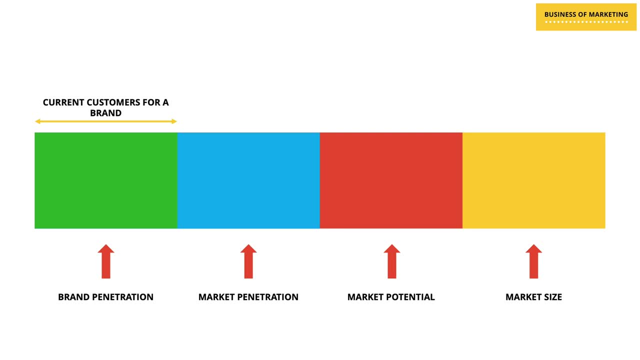 So therefore, 300,000 by 400,000 into 100, which is 75%, And a part of the market penetration is the brand penetration, which is the current customers of the brand, And currently we know that, say, the brand which is the market leader has 200,000 customers. 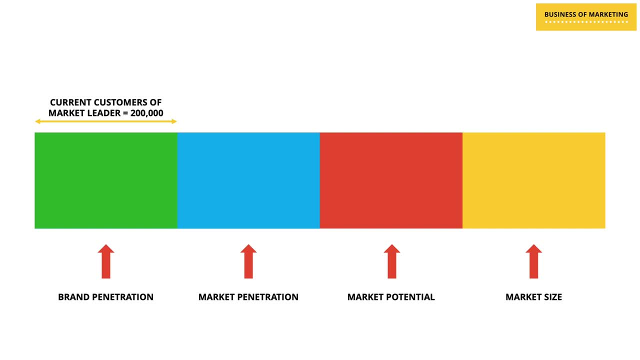 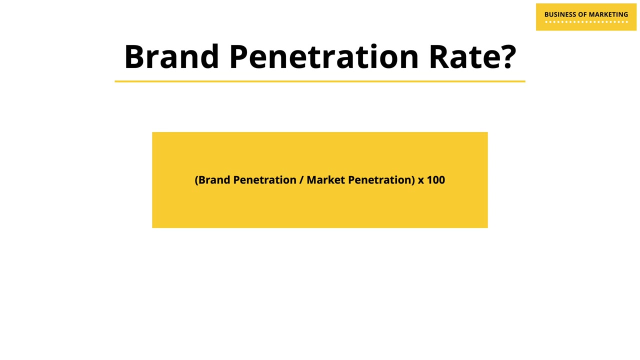 out of the total category customers of 300,000.. Brand penetration rate, which is merely just a percentage of market penetration, we calculated by taking brand penetration, dividing that by market penetration and multiplying that by 100. So therefore, when you divide 200,000 by 300,000 and multiply that by 100, you get 66.67%. 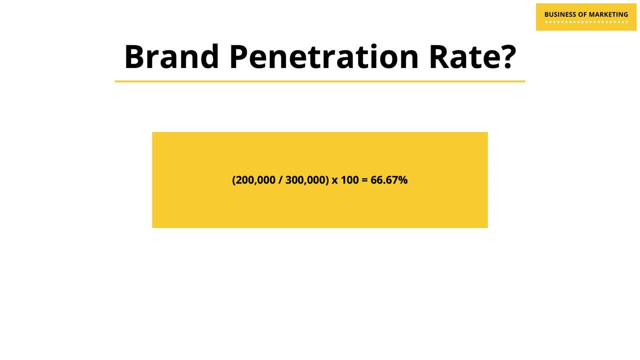 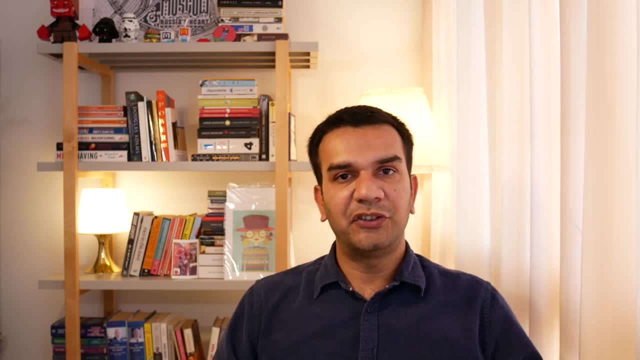 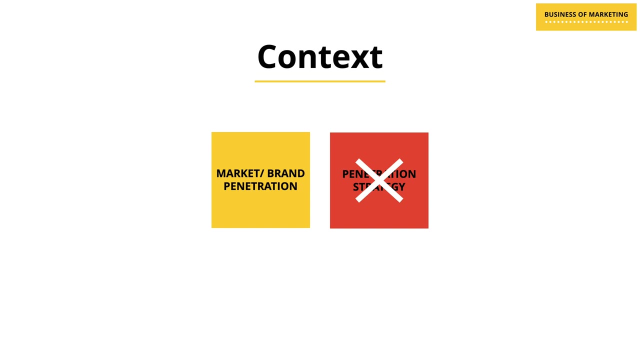 which is the brand penetration rate for the market leader in Singapore. So, therefore, we spoke about a couple of things. Let me quickly clarify each one of those. once again, This video is about market and brand penetration and not about the penetration strategy. I will do a separate video on that. 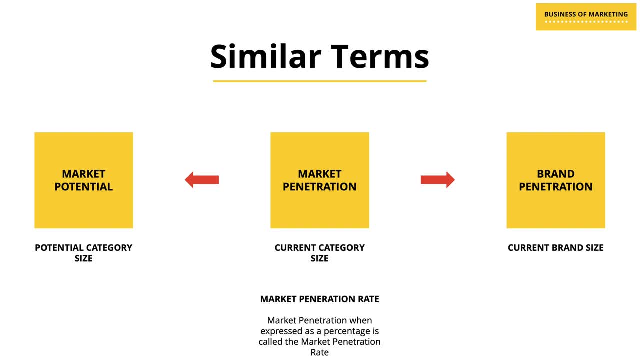 We looked at similar terms like market potential. Market potential is basically market penetration, which is current customers, And when you add the potential customers that could possibly become your customers in the future, you get the market potential, And we looked at different ways to do that. 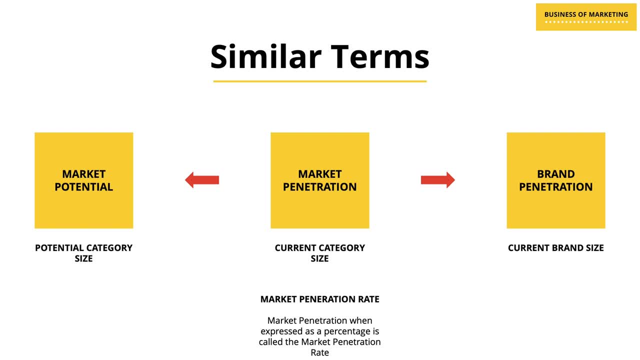 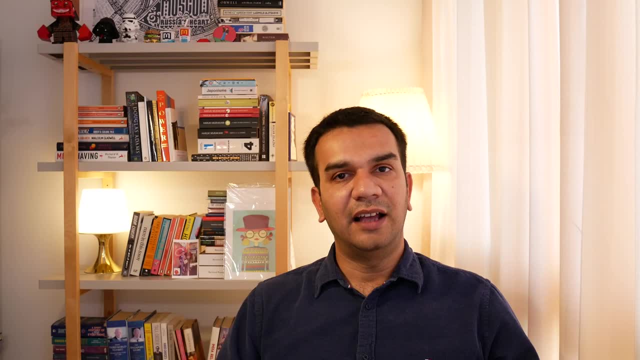 We looked at different ways of calculating the market potential rate, the market penetration rate and the brand penetration rate. That brings me to the end of this video. I do look forward to you joining me in my next video, in which I will be talking about 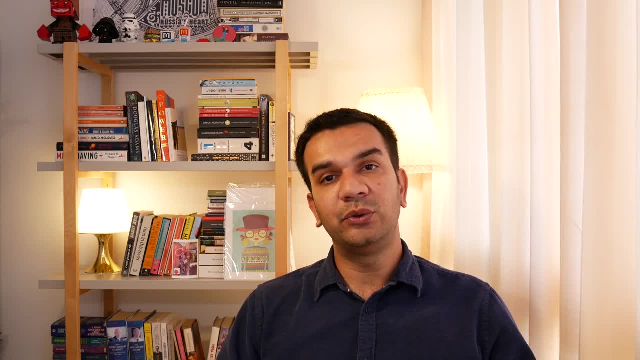 how market and brand penetration data is utilized by marketers in the real world. There are a couple of other terms which are a part of the panel data which they subscribe to. They pay a lot of money for, And we will look into those terms as well. 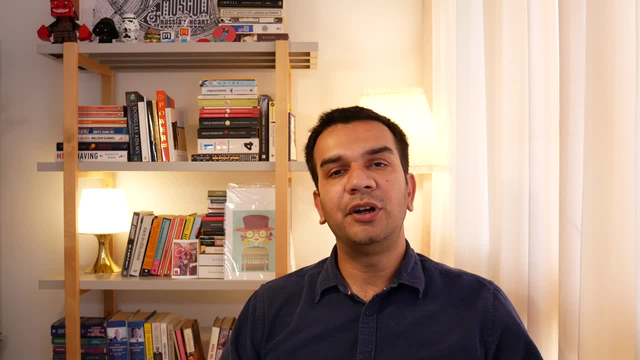 If there is anything in this video that you want to know more about, please leave your comments in the section below And, once again, please do hit like and subscribe to the channel. I will be doing a lot of other videos on marketing and related terms.